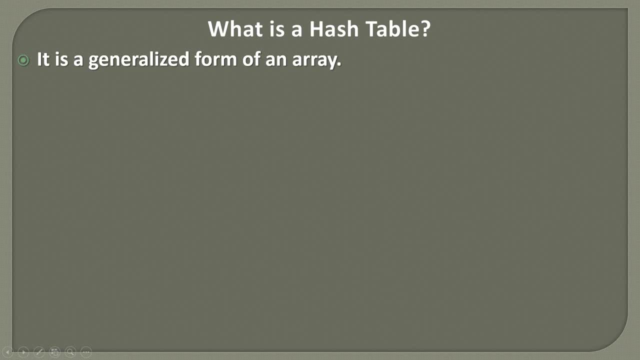 In one of our previous video we discussed that array can be used to store, retrieve and remove an information with a time complexity of one, based on indexes. But we also saw that array had a limitation while implementing the direct addressing strategy via indexes. So we introduced the concept of hashing, Now based on those. 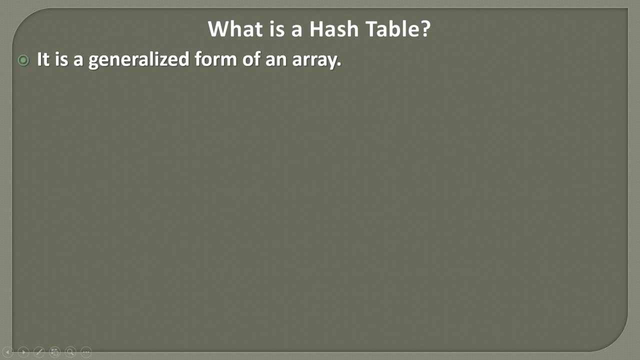 concepts. when we implement a hash table, we basically take a generalized form of an array. So internally, the data structure for implementing hash table is pretty much an array, But it is used with the concepts of hashing and hash function. Now what do we do with the hash table? is the data is stored in the form of? 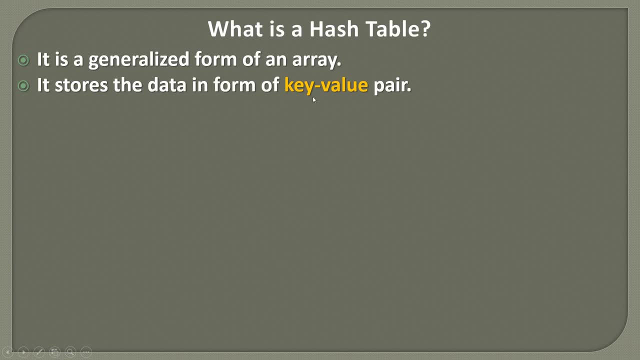 a key value pair. So in our previous video we discussed that how a key is passed to a hash function and an index is returned. So, based on the index, we store this key value pair. So basically, in a hash table we simply put the data in form of key value pair where. 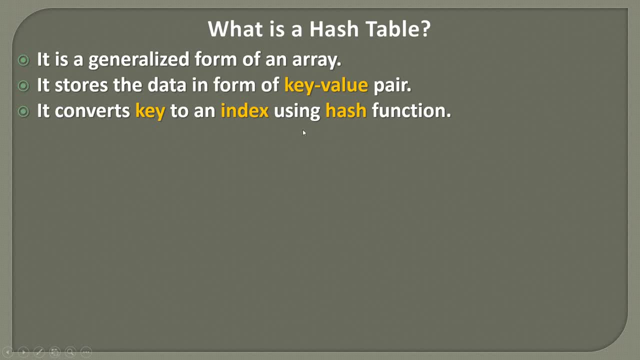 we take the key, we pass it to the hash function And hash function returns an index. So this index is nothing but an index of an array where we simply store our key, value pair, value pair. So this key can be a huge key, But our hash function takes that key and returns. 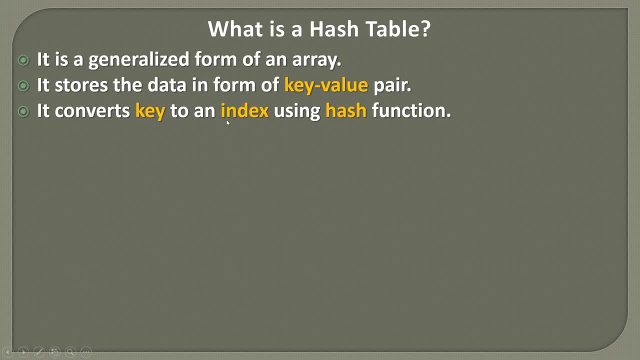 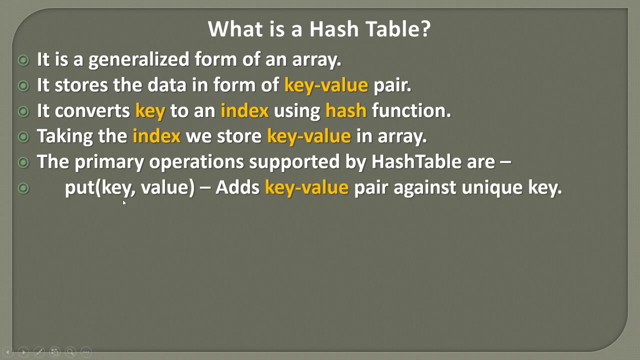 us back a fixed and a small value which is nothing but an index of our array. Now what we do is we take that index and we store the key value pair in the array. And the primary operations which are supported by hash table are: first, is the port which takes in a key. 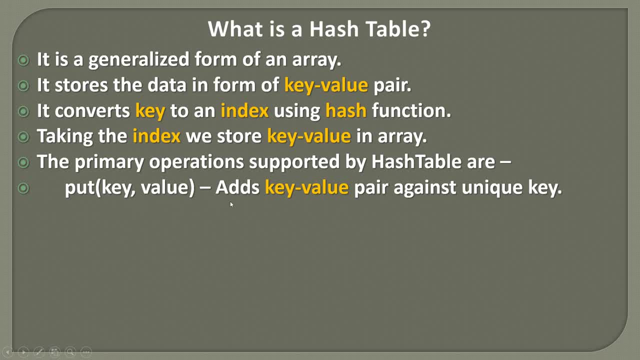 and a value. Now what does this operation does is it adds the key value pair against a unique key. So here our key is unique And if we try to add a different value with the same key, then that value gets updated and the older value will be removed. So here the 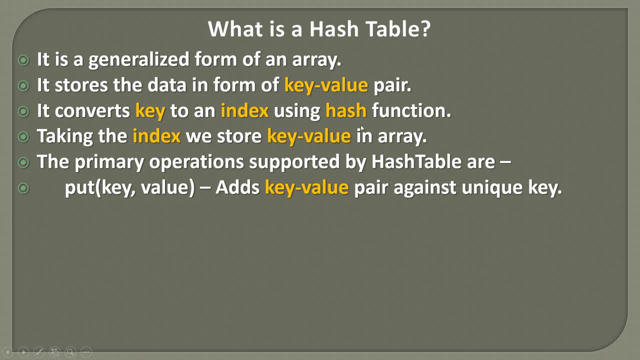 key is unique because this key usually goes into the hash function And based on the hash function calculation our index is returned And on that index this key value pair is stored. Similarly, after storing, when we do get, then the value is returned for that provided key. So here this key goes into the hash function. 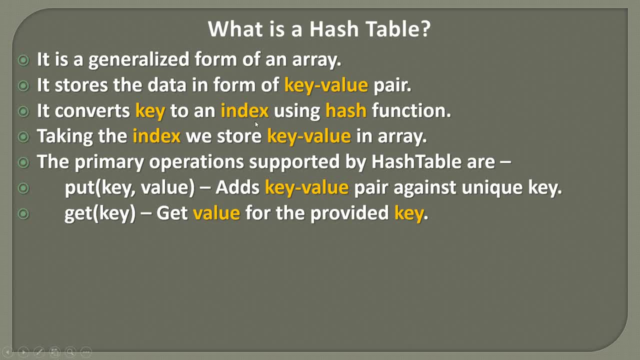 our index is returned And, based on this index, whatever the value is stored in the array, that value is returned for that provided key. So, and the third operation is remove, where we pass the key. So what it does is it removes the key. 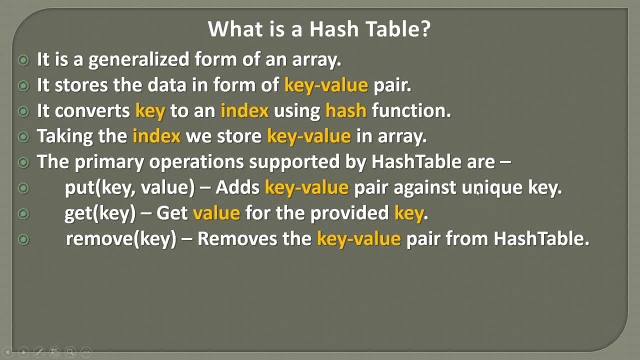 value pair from the hash table. So these are the three primary operations supported by hash table And here, if you see, all these three operations use a hash function And we will discuss all these three operation in greater detail in our upcoming lectures. These all 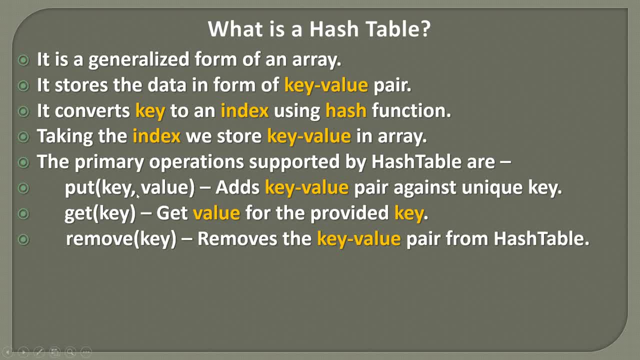 three operation: internally use the hash function, which takes in a key returns as an index and based on the index, put, get and remove operations are performed. So all these three operations are pretty much fast. The average running time of all this operation is O of one. 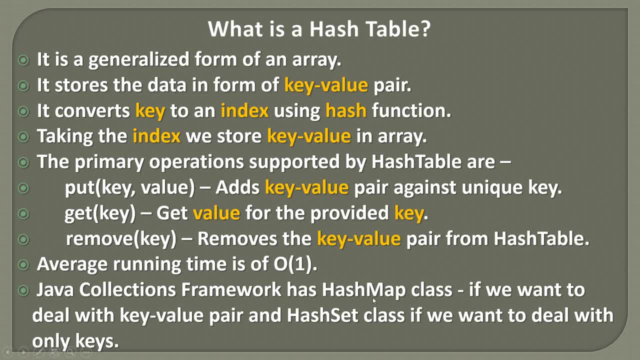 And if you see, in our Java collection framework we have a HashMap class which is pretty much same as the hash table class. So if you want to deal with key value pair, then we simply use HashMap class, And if you want to deal with only keys. 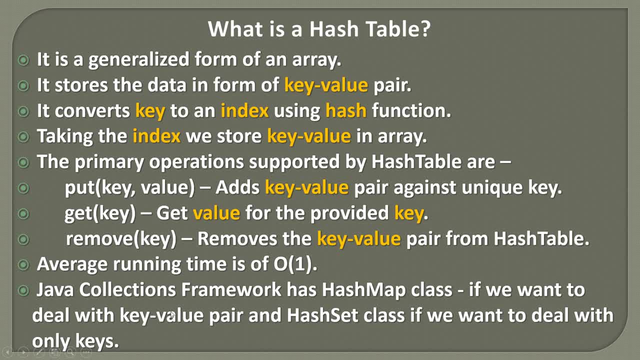 then we use hash set. So here, if you want to store any data in form of key value pair, then we simply take the help of hash map class in Java, which is nothing but an hash table. But if you only want to deal with the keys and not with the value, then we simply use 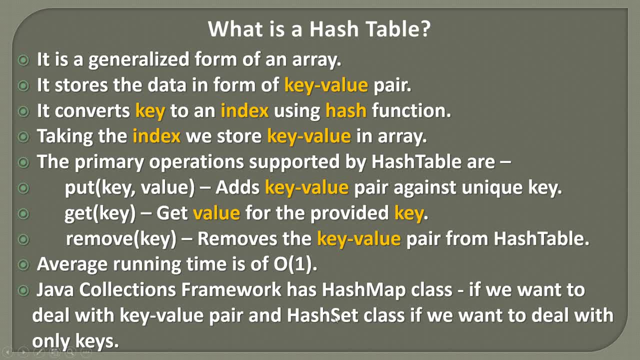 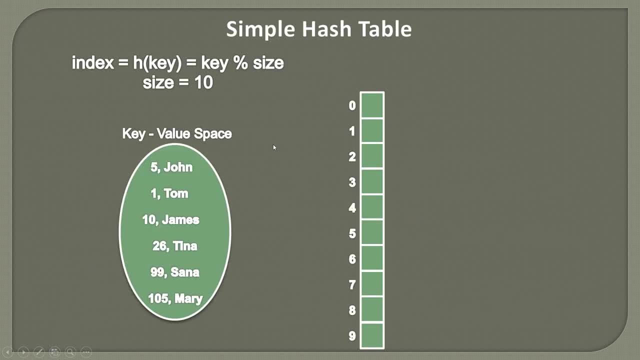 the hash set class, And the idea behind both the classes- to store the keys- remains the same, which we discussed here. So for let's see a simple hash table where we are provided with the hash function as key mod: size, and size is nothing but the length of this array. 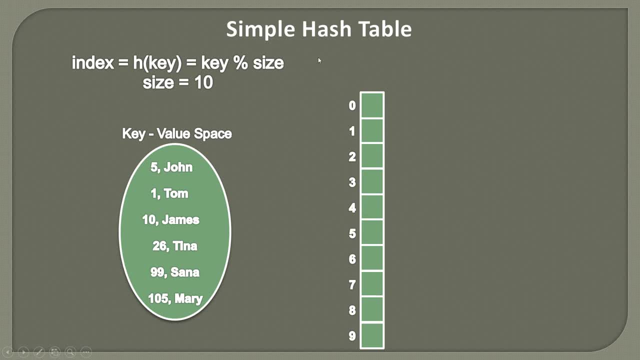 So this array is the internal data structure to implement a hash table. So we simply call it a hash table only Now let's say if we want to store these key value pairs in this simple hash table. So what we do is, let's say, keys. 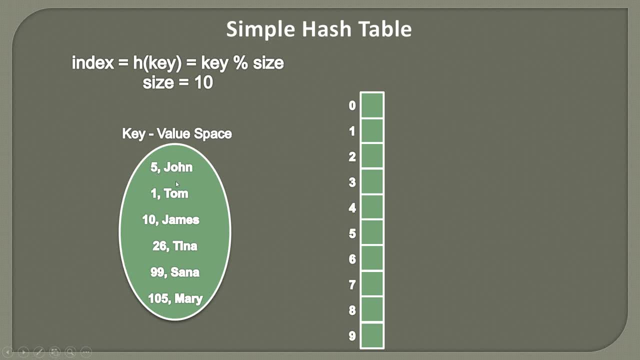 five, five and the value is john. So when we try to store this key value pair in a simple hash table, what we do is we take the key, we pass it to hash function And this hash function returns as an index. So we simply go to that index and store this key value. 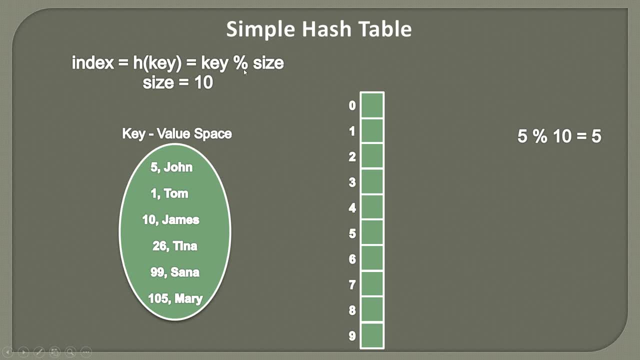 pair. So, for example, five mod 10.. So when we divide five by 10, we get remainder as five. So this is our index, which is being returned by the hash function. So here we simply go to the fifth index And we simply 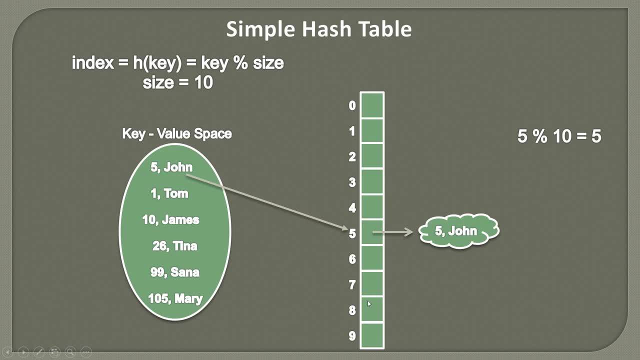 store key value pair. So this array can be taken up as array of key value pairs, which can be our own type object which takes key and a value. Now, if you want to store one comma, Tom, so one divided by 10 gives remainder as one. So here we go to the first index. 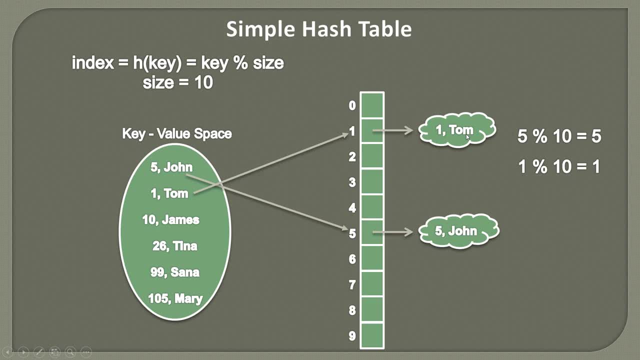 And we store one comma Tom. if you want to store 10 comma James, we do 10 mod 10.. So we get remainder as zero. So we go to the zeroth index and store 10 comma James. there For this key value pair we get six as the. 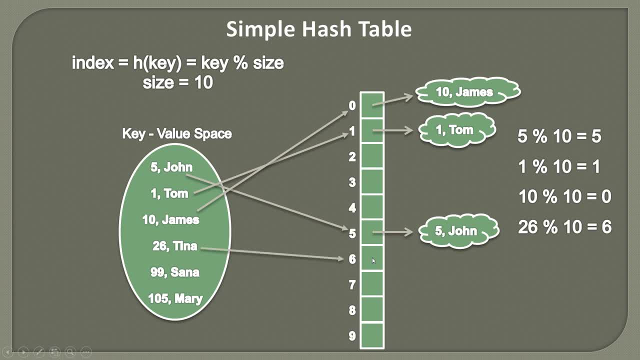 remainder. So we go to the sixth index And we store 26 comma, Tina, For this key value pair. So if we divide 99 by 10, we get remainder as nine. So we go to the ninth index And we store 99 comma, sana, there. Now, if we take the last value, 105, mod 10 will give a remainder. 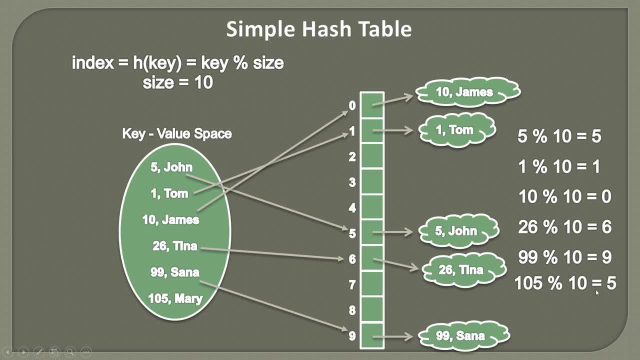 as five. So, friend, this is a simple hash table. So now, here you can see if we try to go to fifth index. here you can see that we already have this value, five comma john. Now the problem is, what should we do with this key value pair? So whenever this kind of situation comes, where we are simply 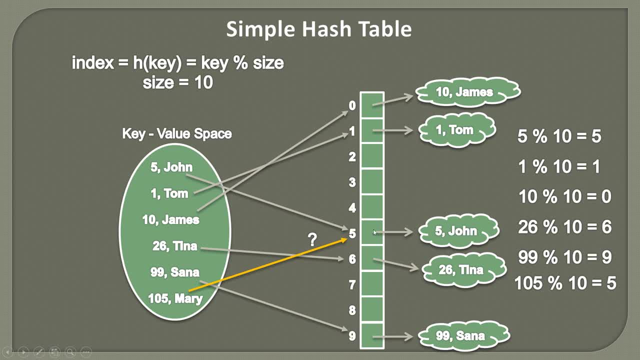 storing key value pair in a particular index and we already encounter a key value pair there. this concept in hash table is called as collision, Because now there is a collision between these two values. that what should we do? So, friends, here you can see that these kind of situation usually arrives when we implement a hash.